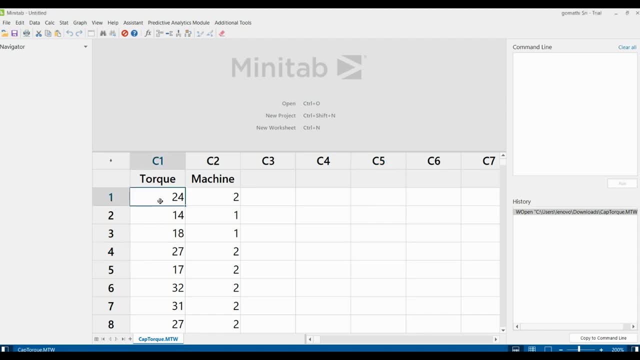 to remove the caps. Here you can find the 68 values. Okay, this is 68 records. we have to check the torque. Okay, and I have two columns. It is a torque and a miscalculation, So I have two types of mission, one and two. Okay, So what is the value for fastening? 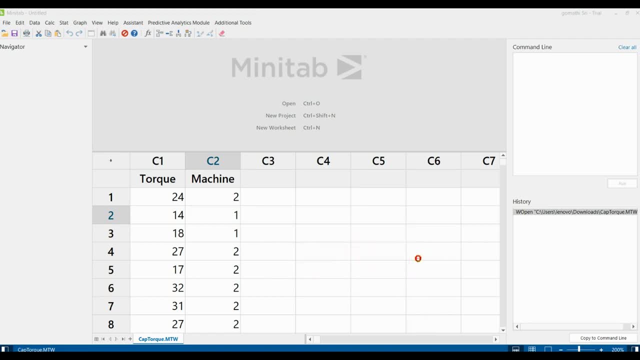 It is 18.. Okay, So as a part of initial investigation, the engineer analyzes the descriptive statistics of the torque measurement to assess the distribution of the data from each mission. Okay, So that is what we are going to do here. See, we have two data. Okay, that is two column, that is. 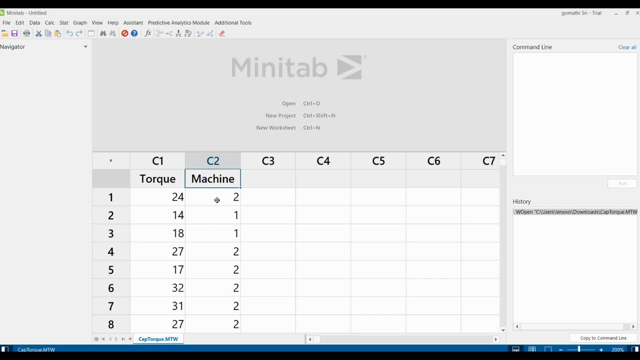 torque and mission. So we are going to find the description of the data from each mission, Okay, So that is what we are going to do here. See, we have two data, Okay, that is two column, that is torque and mission. Also, we have the descriptive statistics for this. So how can we do that? 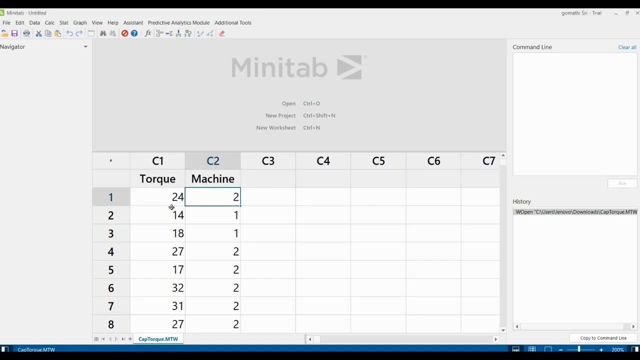 see here. you can see this is a header for both the column and these are all the records. Okay, now I am going to do the descriptive statistics. So click here stat, click here basic stats and stat basics that and click Display descriptive statistics. So once you 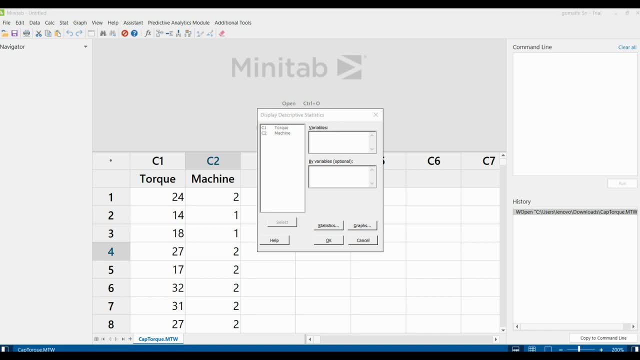 have displayed that. you can see a window. Okay, here you can see that it's a variable you wish to consider and this is by variable. So what is the basic variable you have to use and what is based on? based on which variable? 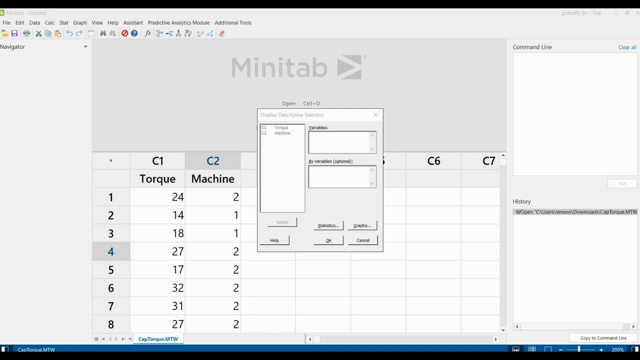 you have to find the descriptive statistics. So in variable I am going to enter the tarq. Okay, so click on the tarq and click select, which will be copied to the variable. Okay, and by variable I am going to tell a mission. 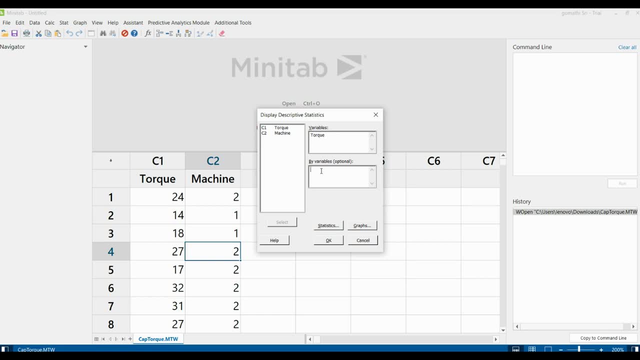 Okay, mission is what my by variable. So I am going to click on the by variable text area and then click the mission and click select, where you can find these two columns: appears in the variable text area and by variable text area. Got it? 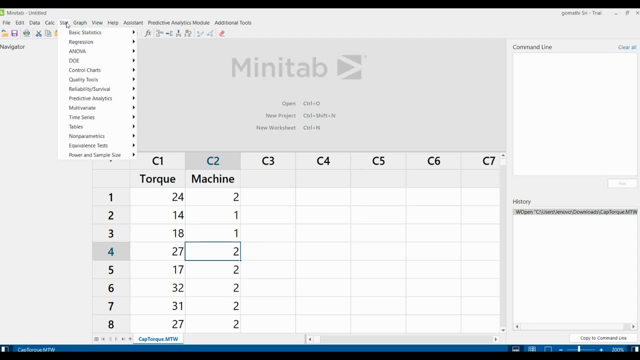 Again I am doing See click on the stat menu and go to basic stat and click display descriptive statistics. You have to give variables, That is for sure. So for that I am giving tarq, because we need a tarq value as 18.. 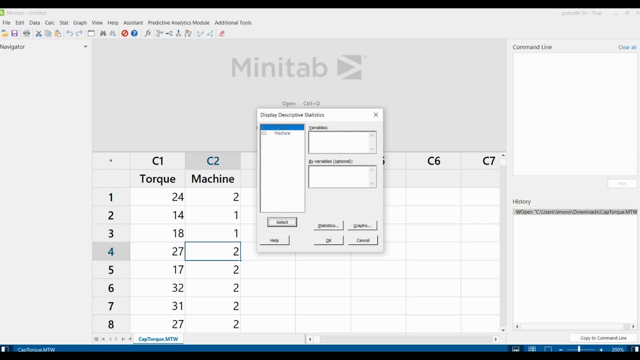 Right, So that is what we have to analyze. So click select. It will be copied in the variable and in the by variable you are supposed to select the mission and click select here. Okay, now we have to decide what are all the statistics: descriptive statistics measure. 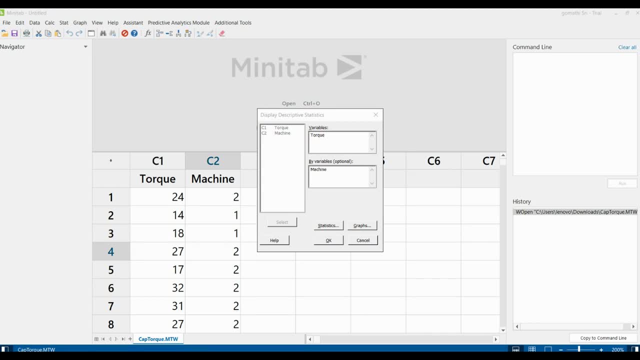 we want. Okay So for doing this. So what I can go with is the. you can just select, Okay. So what I am going to select is: you have two options, Okay: Statistics, graphs. Okay, So now I am going to click the graph button. 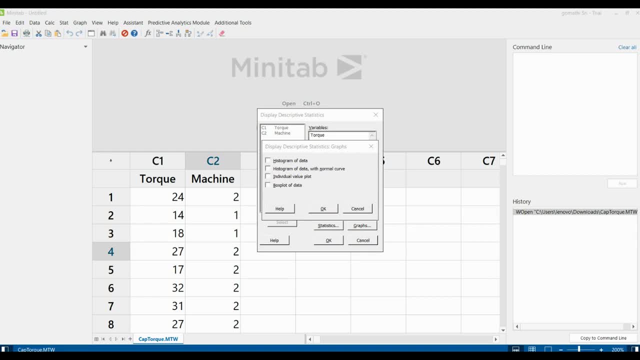 Okay, Let's see the graph button and then I am going to click the histogram of data. You have various graphs. Okay, It can generate various graph. that is histogram, histogram of data with normal cow, individual value plot and a box plot. Okay, 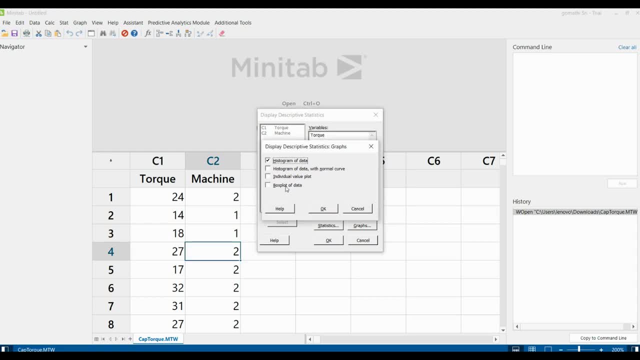 So I am just going to click histogram of data, individual value of plot and a box plot. Okay, Click, Okay. See, you have statistics. If you click on statistics you can see various options that we will come later, and now I am. 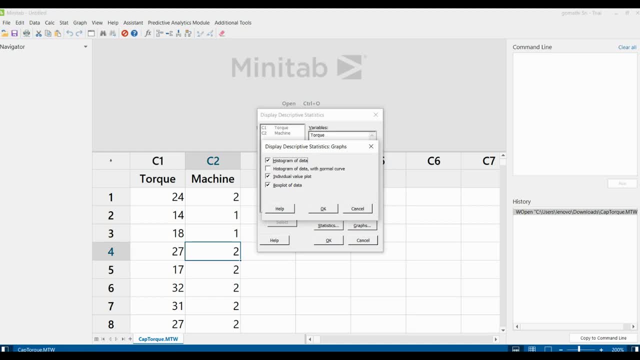 just, I have just used a graph and whichever the relevant graph you want, you can simply select it. If you don't want any graph, you can unselect it. Okay, And click Okay, And then finally you have to click Okay, Okay. 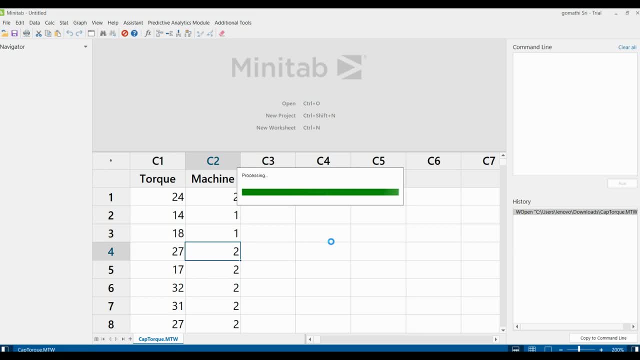 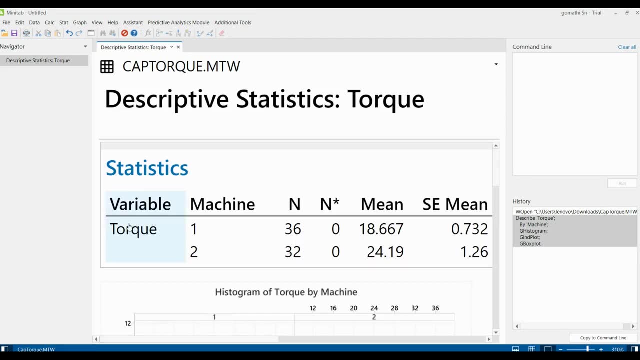 Okay, Once you click Okay, See, it is processing and it will start generating a graph. You can see the graph and the output. Okay, So see, here You can see this is the variable and this is the mission 1 and mission 2: n, that is you. 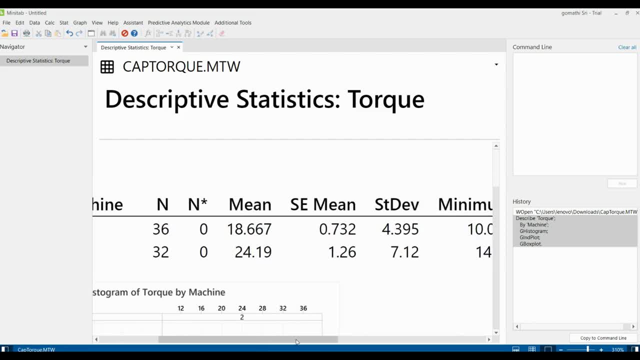 have nearly 62 data Right, So n and 68 data Right. Okay And n. star mean se Okay, Stdve, That is star. Standard deviation: Minimum Quartile 1.. Median Quartile 3.. 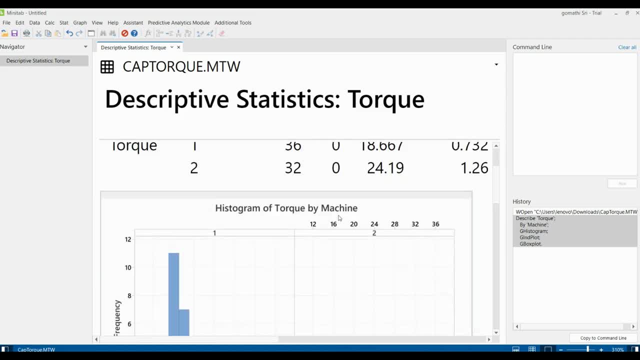 And maximum. Okay, And if you just scroll down you can see the histogram of torque by mission. What is the histogram? And individual value, plot of a torque of mission and box plot of the torque. So these three things which we have given. 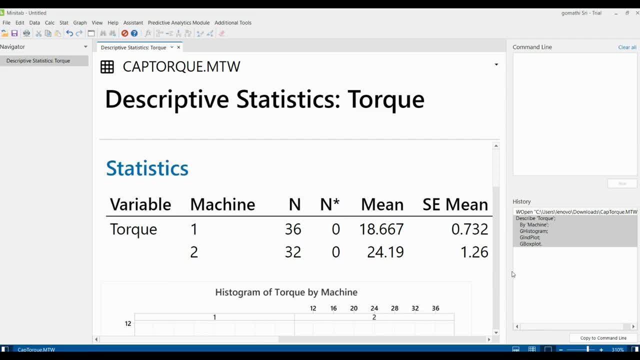 And in the right side you can see that you have the history. So what you have generated, that you can see in the right side. Okay, So here in this you have to interpret the result Right Here. you can see that. 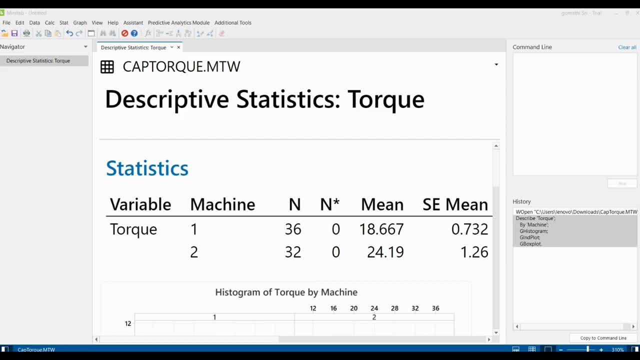 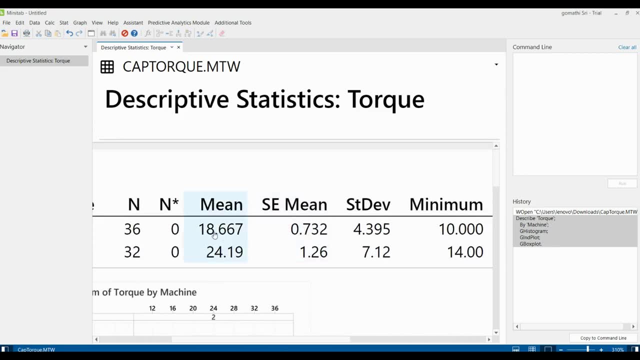 Okay, The mean torque value of mission 1.. That is what is the mean torque value. See you, can you have to? just Okay, This is your mean torque value. So the mean torque value of mission 1 is closer to the target. 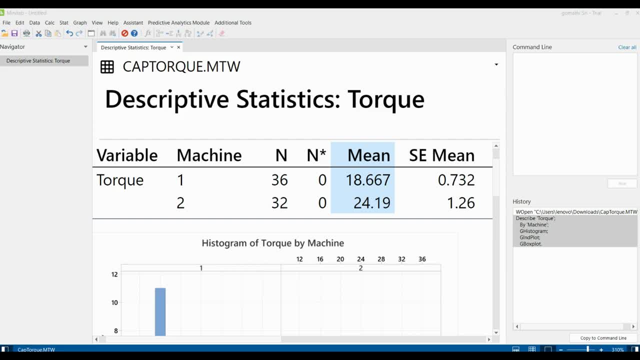 That is what Right. Our target is 18.. Okay Than the mean torque value of mission 2.. Because mission 2 is nearly disjoint, nearly showing 24.19. ok, So the mean torque required to remove cap from mission 1 is 18.667. 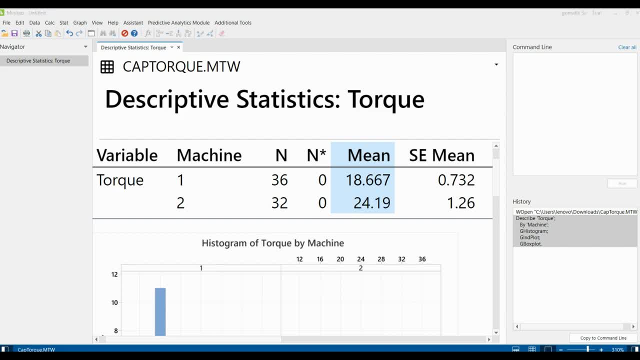 and the mean torque of the mission 2 is 24.19.. So the distribution of data from mission 1 also is less variable and the standard deviation, that is the distribution SE also. you can see standard deviation also. you can see. you can find the various things ok. The graph also shown that. 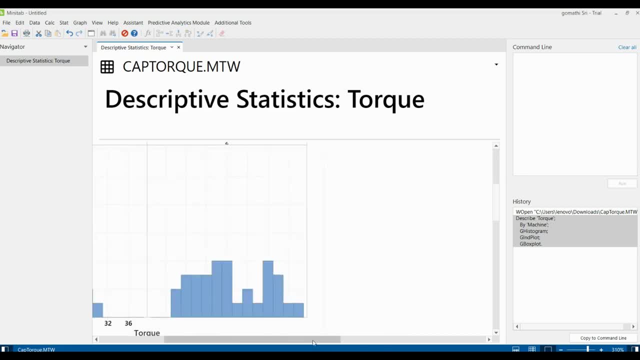 there is a difference in the mean torque. ok, There is a difference in the mean torque that is in C. this is your mission 1.. So it is gradually it is moving around where the 2 you have various difference. ok, So, difference in the 2 missions. ok, So this is what the graph, this is what the 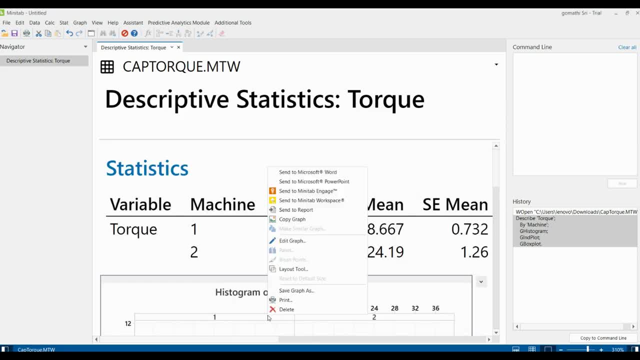 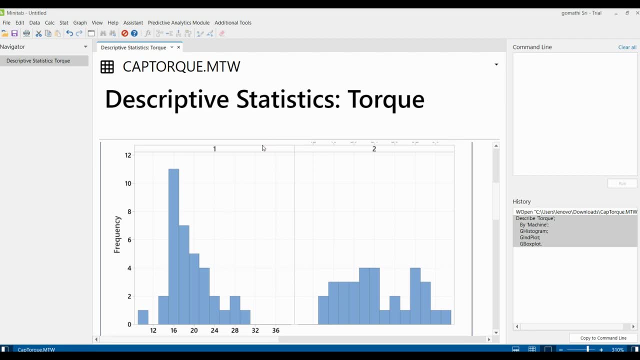 interpretation. you can write it. okay, this is what your output. and see if you just right click on the graph, okay, you can simply copy the graph and paste it anywhere- okay, in your paint or anywhere you can paste it. and if you want to send it to the microsoft word powerpoint, anywhere, okay, you can. 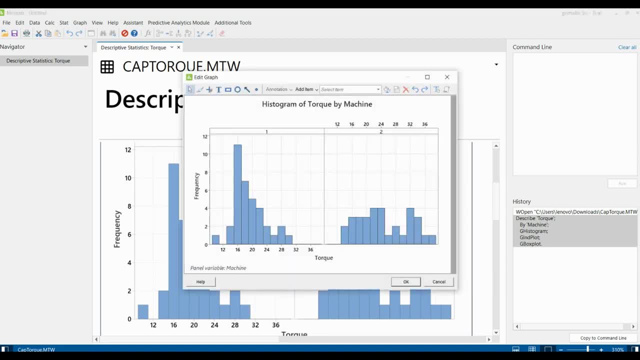 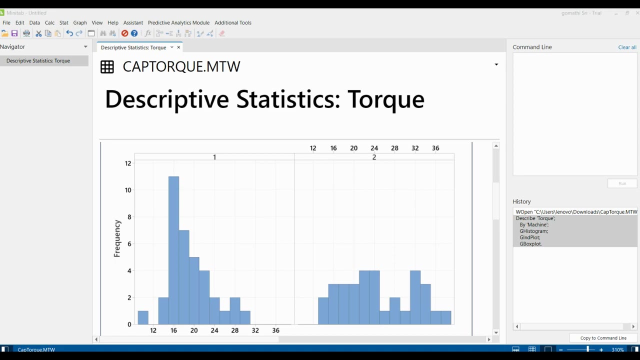 just send it. even if you want to edit the graph, you can click and edit it. okay, if you want to change the colors, you can change, so that we will discuss later in the further session. so this is about what that is. to create the descriptive statistics, that is using the graph. 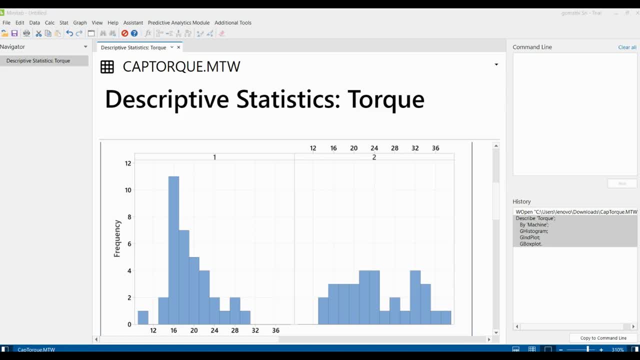 okay, so this is how we have did so. just simply, we have copied the data. okay, the data is already there. so we have used what we have used. we have used only the graph method. now i'm just going to show you how to do it, okay, so let's go ahead and let's go ahead, and let's go ahead and let's. 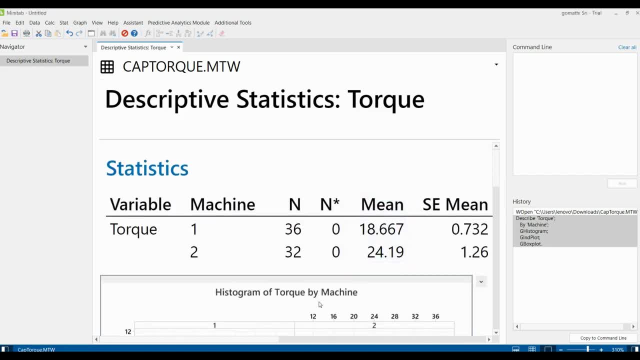 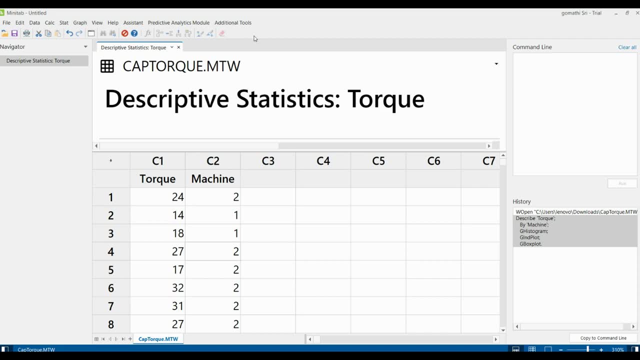 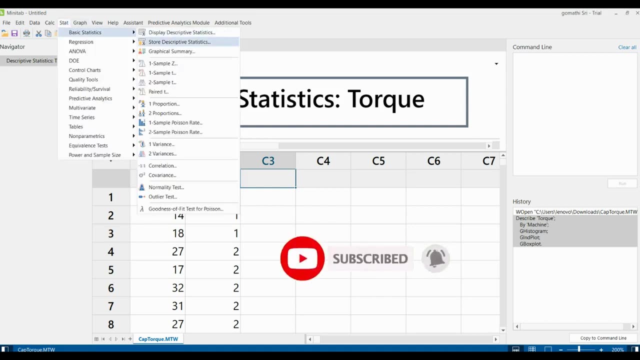 see how to see the statistics like all the other statistics. okay, here you can see that this is a graph method, so i'm just switching over to the normal view using the icon. okay, now i'm going to display the. so click on the stat- basic stat- and you have to click the store descriptive. 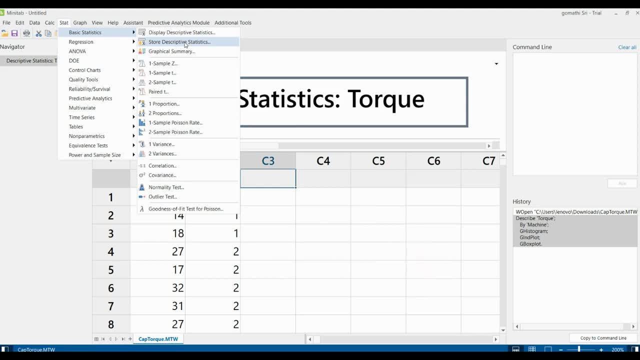 statistics display. descriptive statistics means it will show the output on this display, that is, with the help of the graphs. okay, and if you want to store the value, that is, to summarize the descriptive value using a standard deviation or anything else like a tabular format, then you have to go with the stored descriptive value. so click that and, as usual, you. 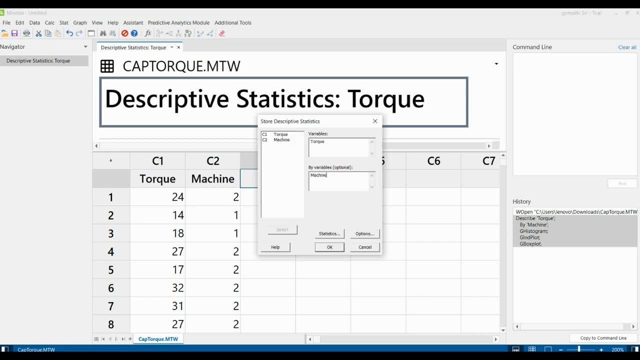 have to use the variable as a tarq and a mission and the by variables and you have to click on the statistics. okay, here you can find various statistics option, that is, the measures which you can give it for. as of now, we are just minimizing it with what see. here you have a. 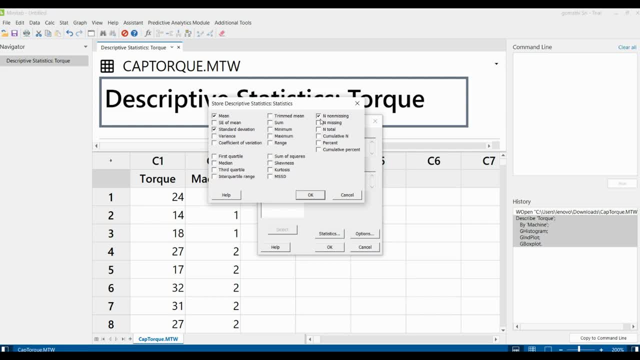 mean okay, and then go to the standard deviation and you have n- non-missing. okay, that is non-missing value. if you want more, you can click see variance. if you want variance, if you want median, first quartile, third interquartile, so whatever you want, you can simply select it. okay, and you can click. 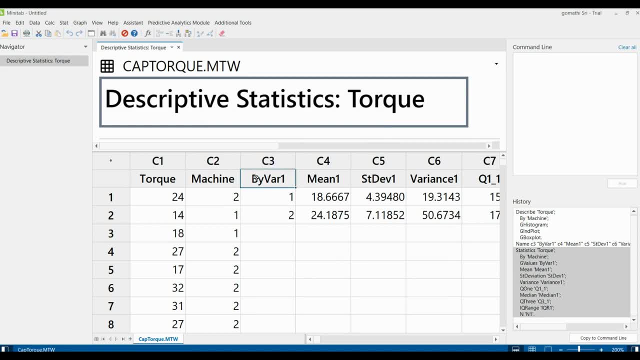 okay, and then finally you have to click okay. so here in the worksheet itself, you can see the output. can you see? yes, this is what the output. okay, so this is your by variable. okay, that is one and two, because this is what the by variable you have given, and what is a mean and what is the standard deviation. so even here you, 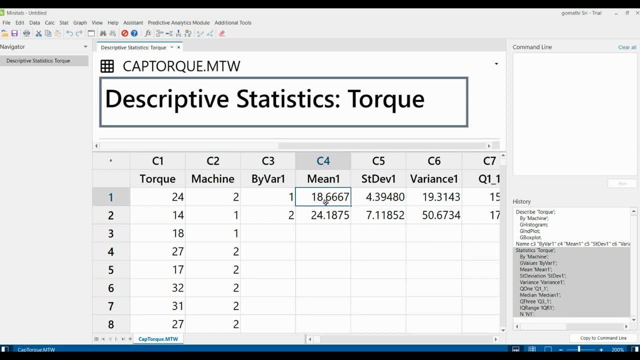 can see. that mean that is for mission 118, which is really equal to the target. okay, that is not exactly equal to the target, but it is somehow near to the target, whereas in mission two it is not equal. okay, and standard deviation variance, you can see it's a, it's a big variance, so you can see.